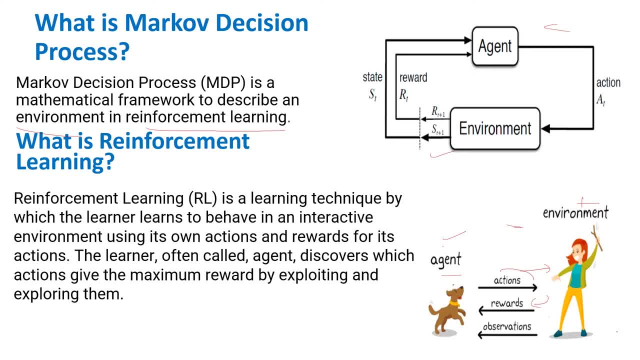 So that is a positive reward and the dog will understand that In case if the dog is jump jumping on, anger on her and it is biting her, then she will show some negative rewards, negative reactions. So then the agent is supposed to align its action depending upon the rewards it is getting. So if 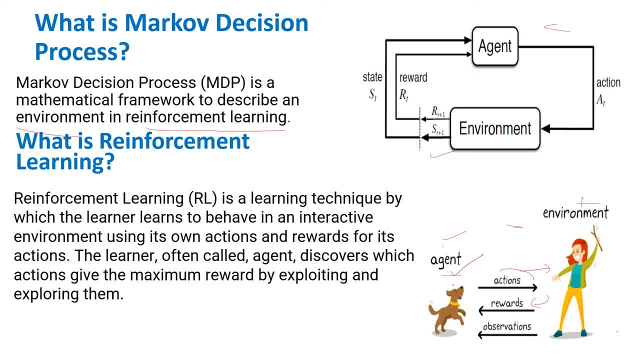 then it will align its actions- right actions- in such a way that it is getting the positive rewards. That's what's the goal of the real-time reinforcement learning agent. So the agent will align its actions depending upon the rewards given by the environment and through that it is going to achieve the goal. it is for what it is designed for. 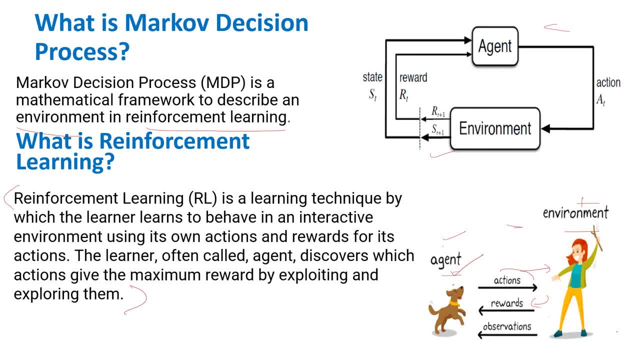 Now we may understand what is reinforcement learning definition: Reinforcement learning is a learning technique by which the learner learns to behave in an interactive environment. So the environment is going to keep on interacting with the agent by the with respect to the action it is showing to the environment. So through the rewards it is going to get back. 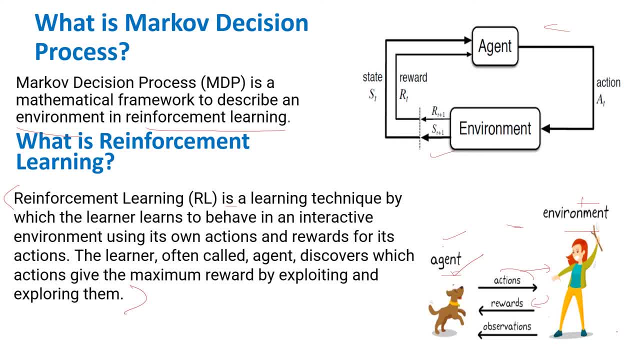 So the learner often is called as the agent which discovers the actions by giving, getting the maximum reward. So the agent is supposed to get the maximum, maximum rewards from the agent, so through which it is going to align its action and achieve its goal. So that's the crux of 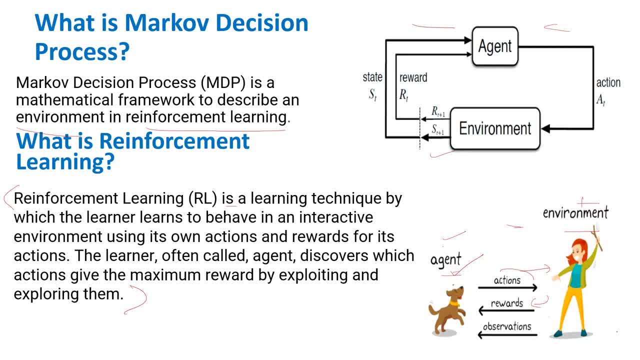 reinforcement learning. Now we will understand this formal diagram. So here in this formal diagram, so we see an agent, so which is which was a dog earlier, and the environment which was the girl earlier. So this environment can be anything as a chess board, or if the agent is trained for. 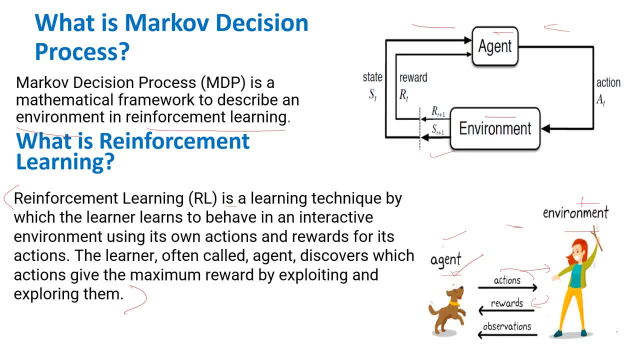 picking an object, then the place where the object is placed is going to be the environment. So we see an ST, that is state, and we see a reward RT, and we see ST plus one, that is another state, and the RT plus one, it's another reward. So we'll understand this. So, when the agent is actually interacting, 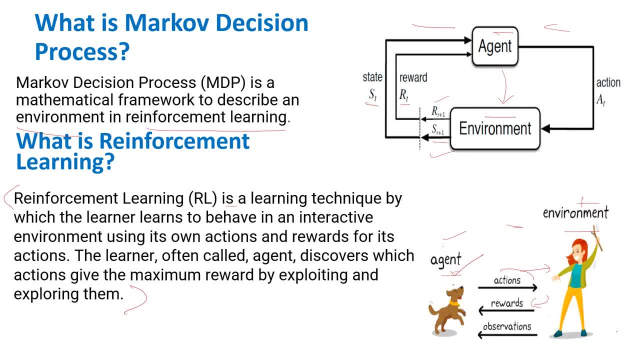 with the environment, so the agent can be in n number of states. For instance, if the dog is lying on the floor, that is one state. If the dog is standing up, then that is another state For each and every state of the, each and every state. 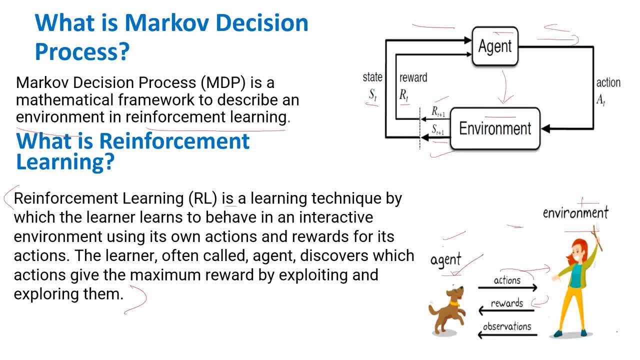 in which the agent is in, it will exhibit certain action A. So with that action A the environment is going to give some reward and with the reward it gets, it is going to either stay in that particular state and keep exhibiting that action or it will transit to another state. ST plus one. 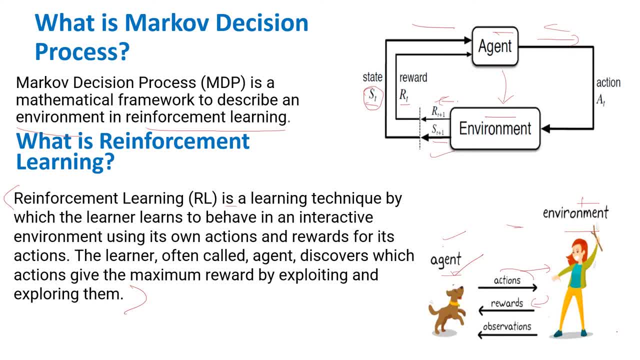 and it will choose some other action which is from that particular state. So this is going to go again and again till the goal is reached. That's how reinforcement learning works. So reinforcement learning should be understood as Still, we may not able to. we may not be able to. 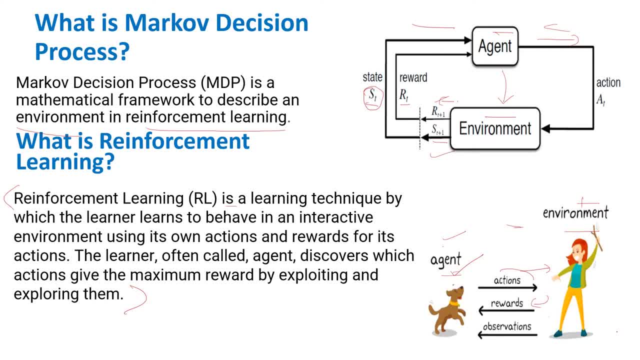 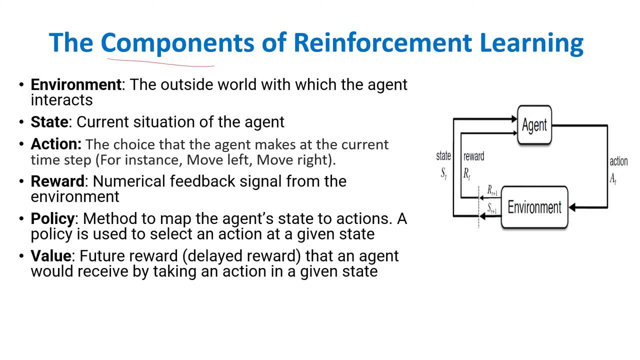 understand the Markov decision process. that's fine. So we'll gain clarity as and when we move on. We'll have a closer look of about the components of reinforcement learning. So the first component of the environment, we already saw the girl who was having the stick in her hand. So the any outside. 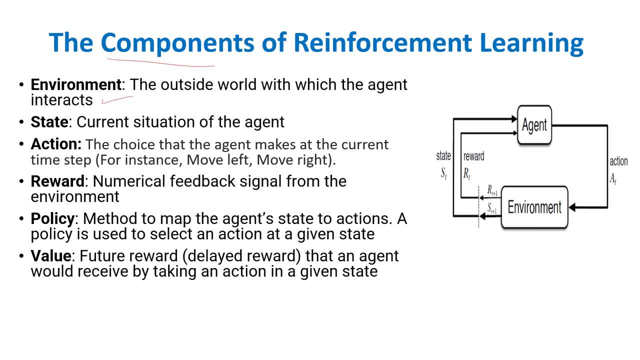 world, so which is in which the agent is interacting to achieve a particular goal, that is, the state. So, while interacting with the environment, so in the process of achieving the goal, So, for instance, playing the chess against a human or picking up a job, the agent can move from one. 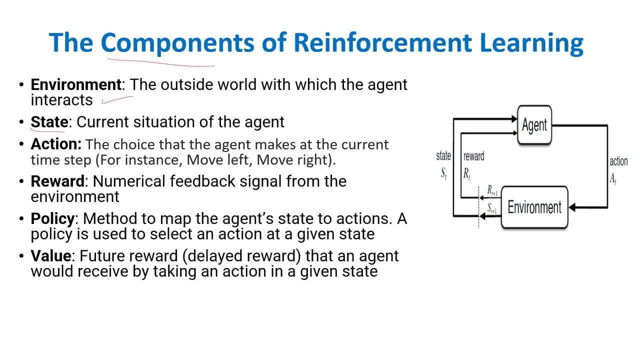 state to another. It can show itself, in exhibit itself in many other states. For instance, the robox sitting in a chair is one state, standing up another state. so it is in the process of goal. so, while in, while, while doing this, while in getting involved in this process, it can be in a 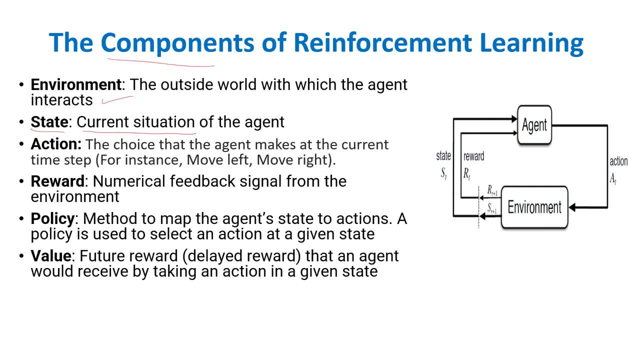 number of state, so primarily the current situation the agent is in, so at present it is in, so that is called as a state the action at each and every state s. so it might choose any action. so for instance it can go up, it can go right, it can go down, it can go left, so there are n number of 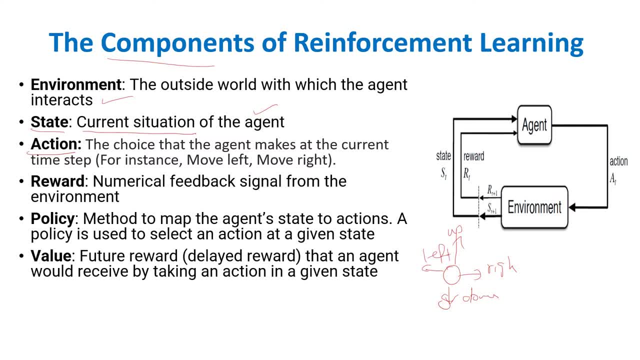 actions that it can opt to choose. it can opt at a particular state. so that is an action, the choice of agent it makes at particular time step. that is the action, the reward. the reward is primarily the numerical value that is got from the environment. so for each and every right action, 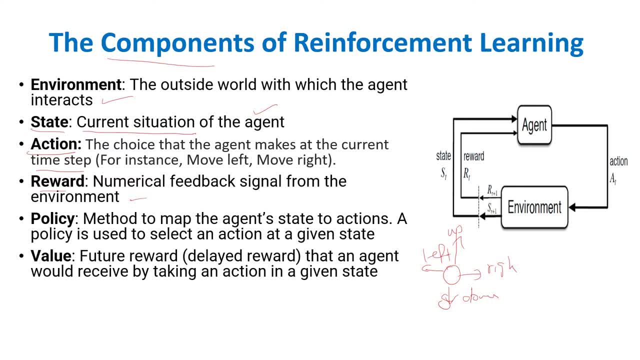 and the state transition it takes, it is going to get a positive reward. so the goal is that it has to get the maximum number of rewards. through that it is aligning its right number of actions and through that it is achieving the goal for which it is designed for. so that's the idea. 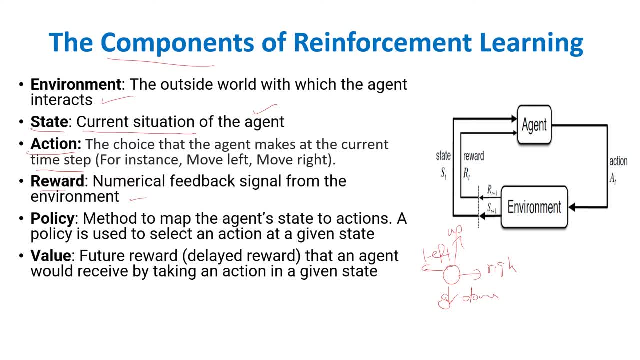 policy. policy is nothing but it's a function. so that is used to map the agent state to action, though it is in this particular state s, and it can move to another state, st plus one, so while moving. so it can choose either of these actions to this state. so the policy is nothing but while. 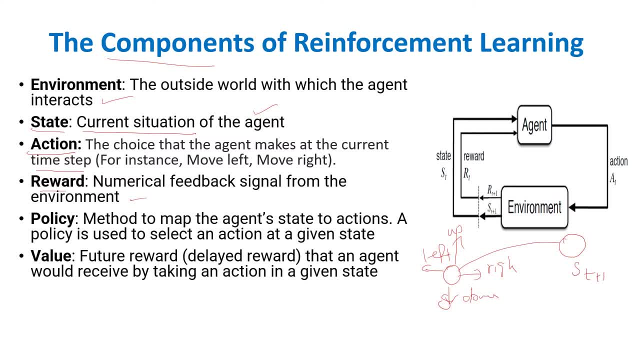 taking a transition from one state to another. what? what are the action? what is the action it is taking so it is not only constrained with these two states? the agent might transit to n number of state till it reaches the goal. so for, at each and every state, what is the right action it is taking so that it 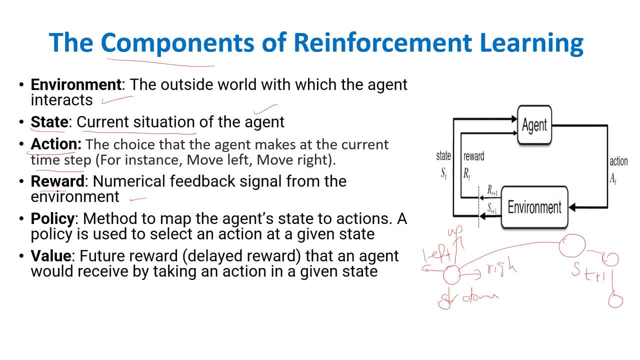 is maximizing the rewards while in the process of achieving the goal. so that is the policy. so what we are interested in finding is that, at each and every state, what is the right action? it is supposed to be taken. so the what is a set of actions that is to be taken at each state. so 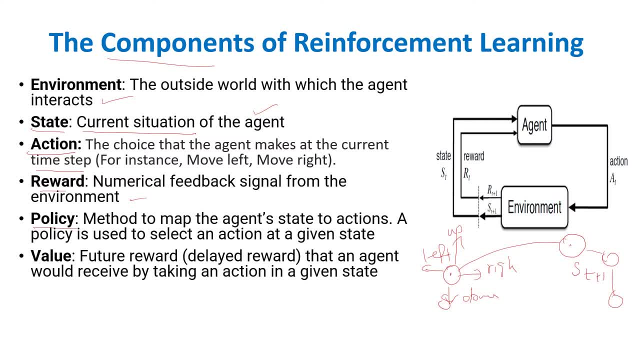 that is called as a policy. okay, so the value is nothing but the future reward. so value is given to the state. okay, so the value is the function, that is, the value is given to each and every state. so each and every state is going to get a value. so that 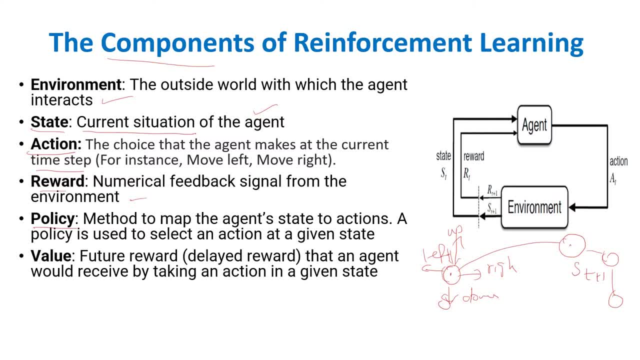 the when an agent is transiting from one state to another. for instance, this is a state is having some value. the agent will only decide to shift to the state depending upon what is the predicted return it would get if it transit from this state to this state. so that is called as the value. 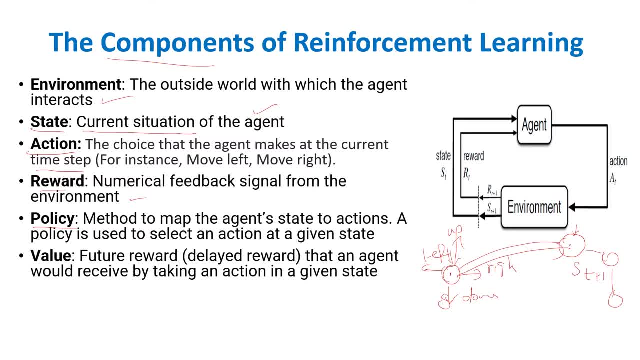 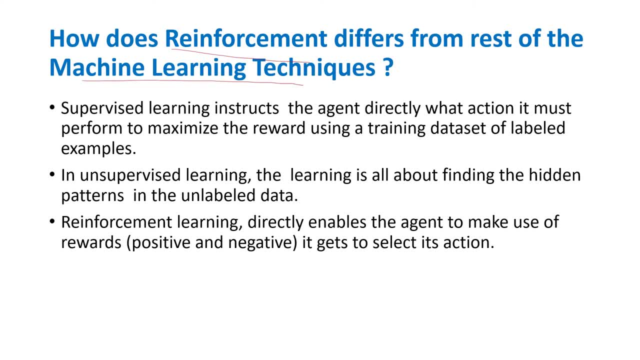 okay, so these are the components of reinforcement learning. okay, so the reinforcement learning is also a type of machine learning technique, so we should understand that. like what? how does it differ from the rest of the machine learning techniques? a supervised learning? so it's also one of the machine learning techniques in which we have labeled a training data set. so we have 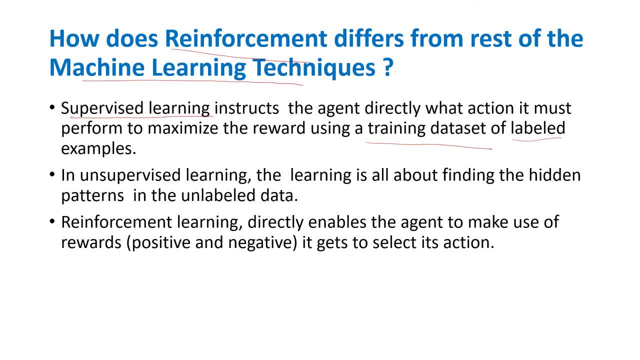 a labels, for instance for an offer. for example, when we are building a classifier which is supposed to classify the dog pictures and the cat pictures. okay, so when a dog is shown dog picture is shown, it should classify that as a dog. when a cat is shown a cat picture is shown, it is, it should. 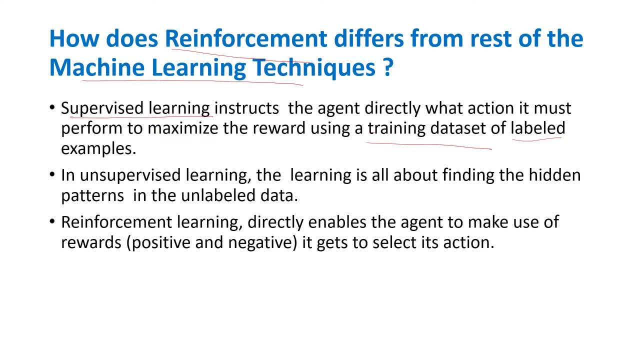 classify it as a cat. let's say we are building such a supervised learning model, then the we would have already got the training data set which is labeled. so that means the cat pictures are all are tagged as cat and dog pictures are all tagged as a dog. so with these tags and the dog pictures and the cat pictures, it is associating with the. 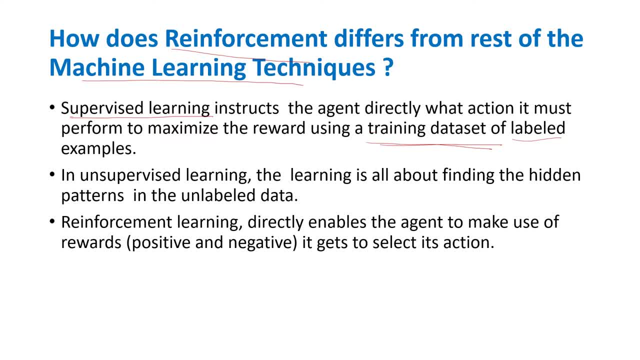 labels and the features of the dog and cat pictures and it is coming to a conclusion and it is building a model so that whenever a cat picture is shown, so without a tag, that it is without the label, then it will automatically classify that it is a cat and uh respectively. 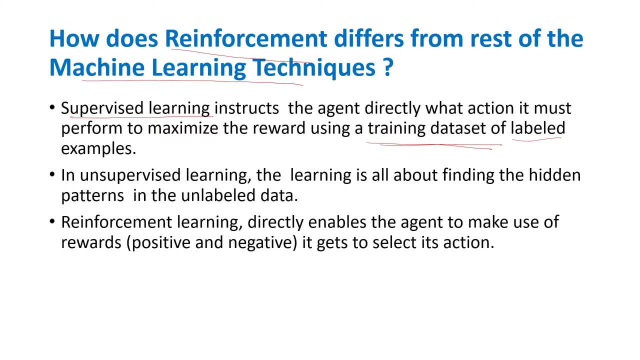 the same for the dog picture. that is supervised learning. so, with the labels and associating that with the numbers of the data, that is, the pictures or the pixels, the pixels are going to be the features. then that is supervised learning. the unsupervised learning, on the other side, will not have the 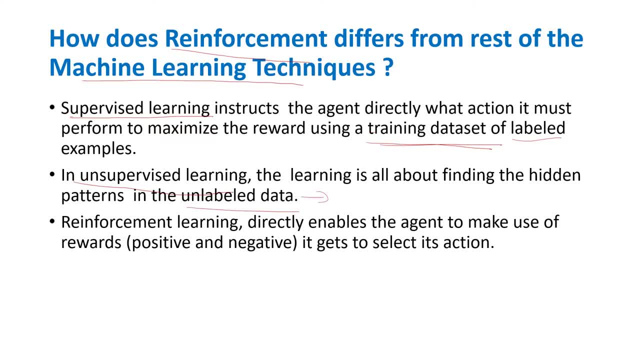 training data will not have the labels, the dog pictures will not be having the label, but still it will do some grouping so that we call it as clustering. so it is as simple as like: for instance, we have apples and oranges. a baby tries to cluster it. uh, based upon the 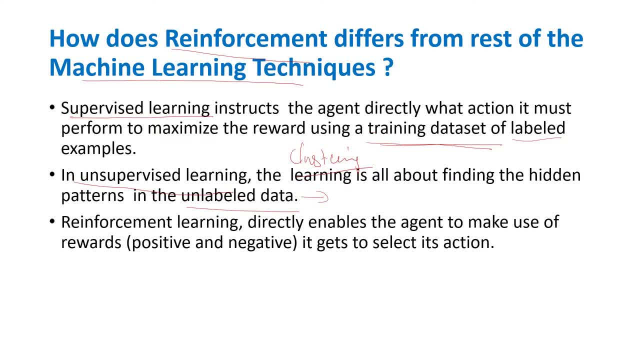 color of the fruit and the shape of the fruit. so, without knowing the labels, we are grouping based upon the similarity of the features of the data. so that is unsupervised learning, the reinforcement learning. on the other side, it is reaching its goal depending upon the positive and 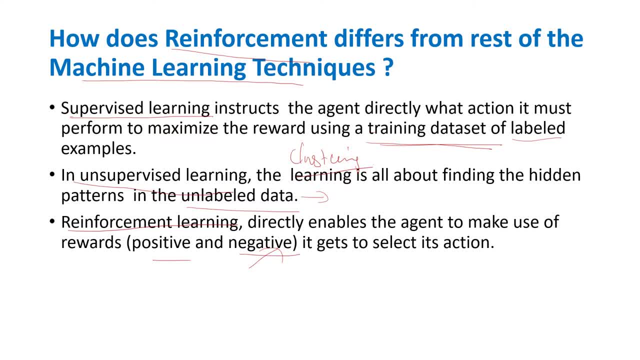 the negative rewards it is getting from the environment and it is aligning its sequence of actions it takes and while shifting from one state to another. so that is reinforcement learning and that's how it differs from the rest of the data, the machine learning techniques as well. okay, so now our goal was to understand. 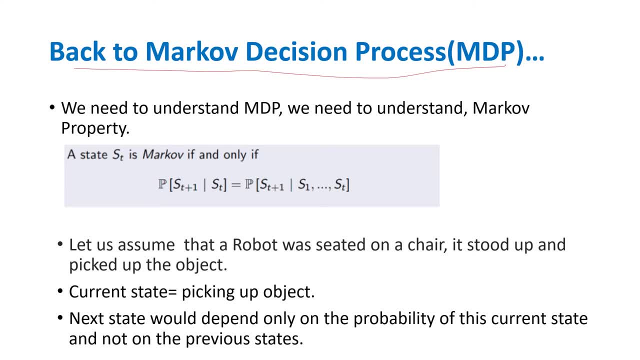 Markov decision process. so before even we understand Markov decision process, we need to understand what is Markov property. so Markov property is all about, like state transition probabilities, understanding state transition probability. a state s st, so here it is st. so a state st is Markov if, and only if, 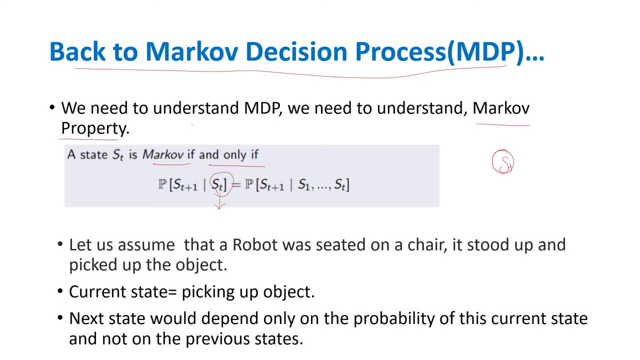 given we are in state st, the probability of the transition. so when the state transition is taken from st to st plus one. so this, the the probability of going to this state, is only dependent on the probability of this particular state st and not on the earlier states. so we 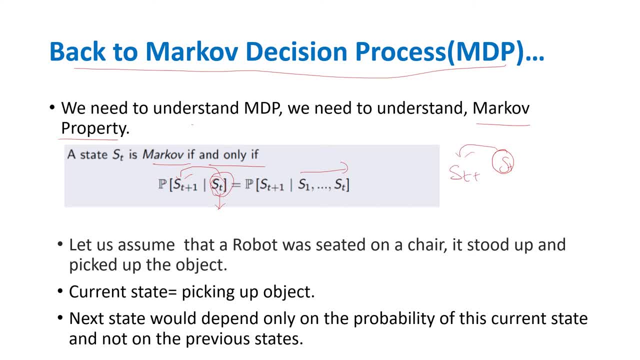 before, before shifting to st plus one from st, there could have been n number of states, so t minus one, st minus two and so on. but we are not bothered about the probabilities of the earlier states, we are only bothered about the probability of the current state, the immediately previous state. 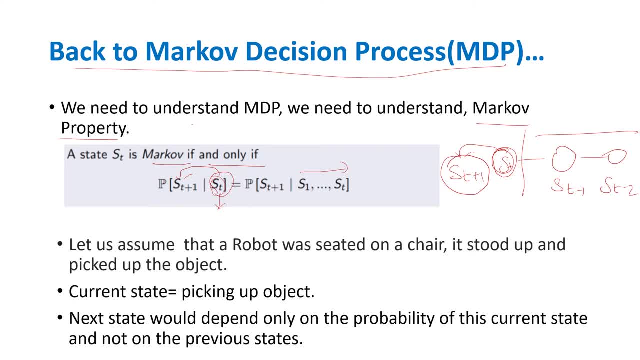 so to predict the probability of the next state. for we'll take an example to understand this better. so let us assume that the robot is seated on a chair- okay, that is one state. it stood up- that is another state. and it is picking up an object- that is another state. so the current state is: 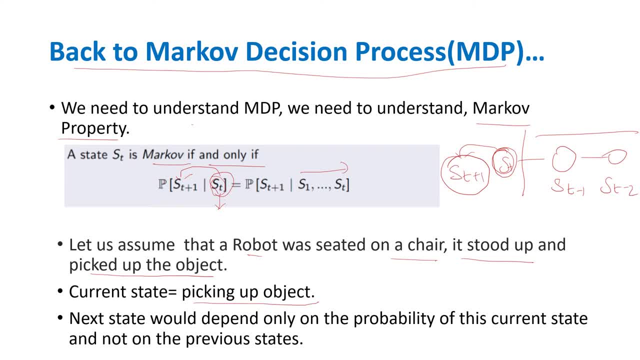 to be understood as the picking up the object. it is having some object in his hand. that is the current state, the prediction of the robot taking the other state. okay, so that is dependent only on the probability of this particular current state and not on the probabilities of these states. the 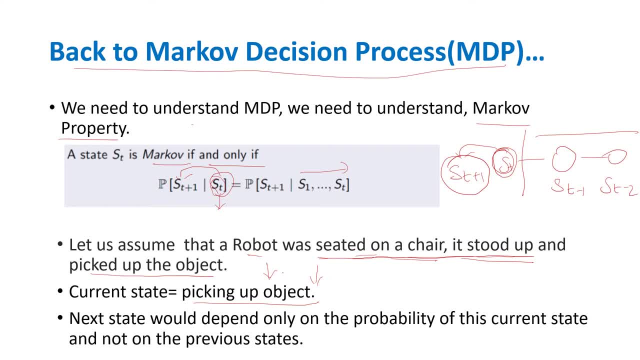 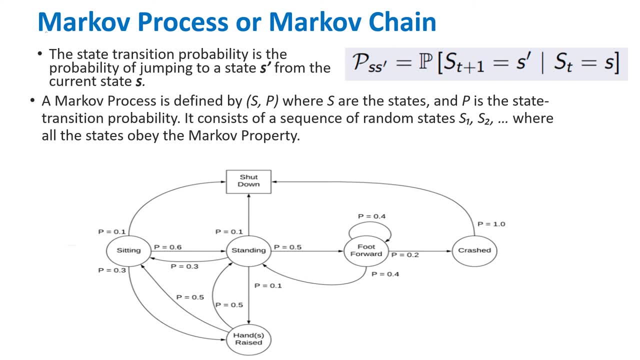 earlier states. that is about the Markov properties, so this should be understood first. okay, so we have not still understood Markov decision process, so before that, we will understand what is a Markov process or a Markov chain. okay, so you see a state transition diagram here. so this is what a Markov process. so these are the states. the circle ones are the. 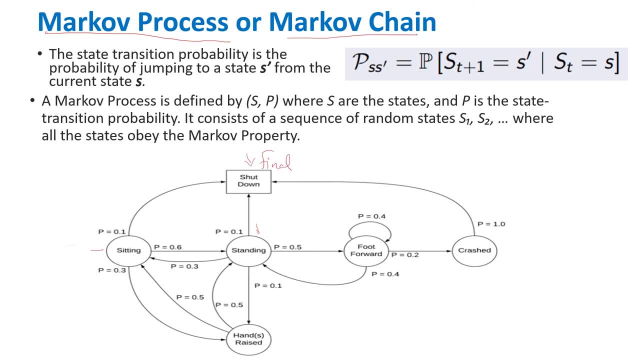 states. even this is a state. this is the final state. okay, so these are the states, and why we call this as Markov chain is that we are going to loop, repeat the process from one state to another. so again and again, so we can be in sitting state and we can transit to standing state and we can 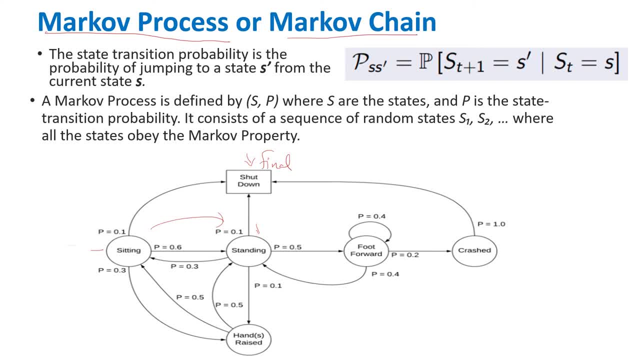 move from there and then we can come back to the sitting state from the standing state. so this is going to do go again, and again, and again. but there are numbers associated, you see that. so this is a probability. so, for instance, we'll focus this particular state. 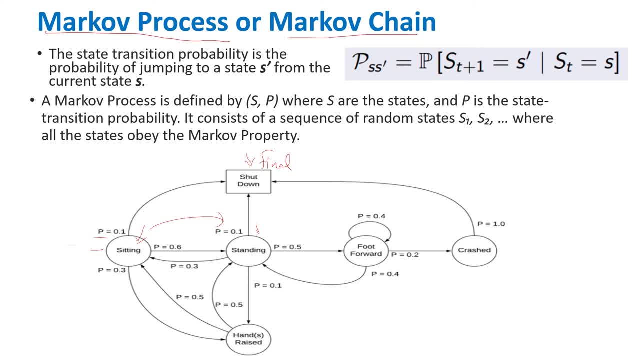 let's say the robot is in the sitting state. so the probability of the robot transiting from sitting state to standing state is 0.6. that's what it's shown here, and the probability of the robot shifting from sitting states to the shutdown state- the final state- is 0.1. it's very less. 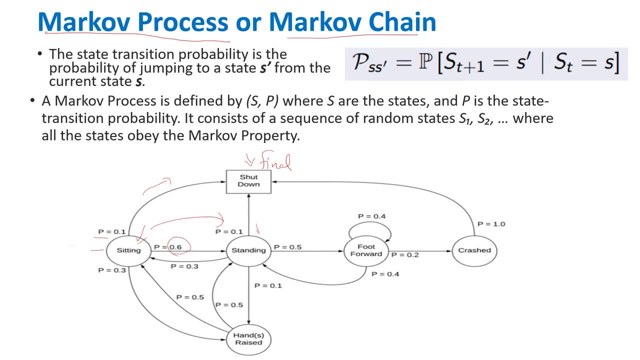 and the probability that a robot can raise its hand from the sitting state is 0.3. so these are the probabilities of the state transitions from this particular state. so if you look closer, when you add up all these probabilities, that is emerging out of the state. 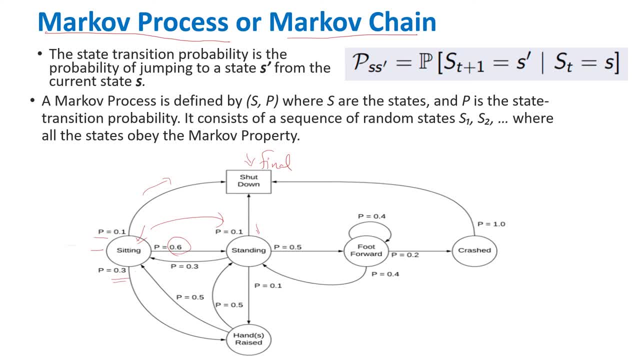 that 0.1 plus 0.6 and 0.3, they add up to 1, because if we are dealing with probability, it has to add up to 1. so this is the state transition probability: what is the probability that a particular state? 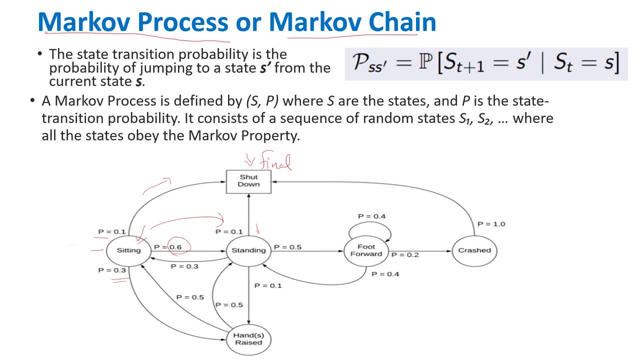 will get transited to another state. so that's what Markov process is and we have to remember the Markov property that we saw earlier. so the probability that the probability that the robot will transit from sitting to standing is only dependent upon the probability of this particular state and not on the earlier state in which the robot was. 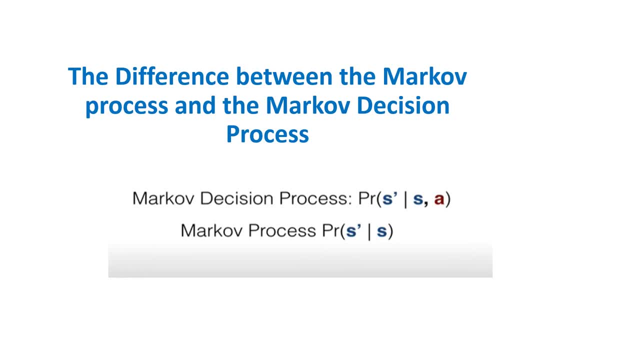 okay, so now we haven't seen Markov decision process yet, we have only seen the Markov process. this is an exact difference between the Markov process and the Markov decision process. you see an additional a here in Markov decision process. so Markov process only tells us what is the 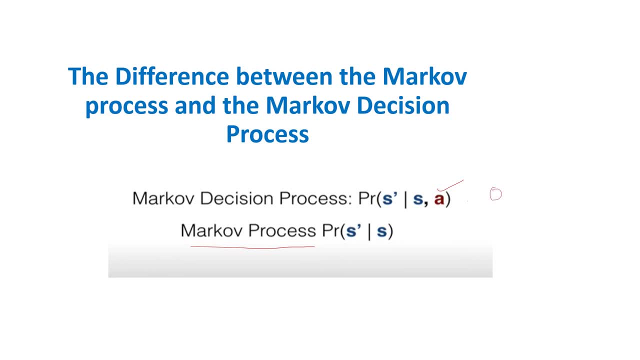 probability that a robot will transit from sitting to standing state, to the shutdown state, will shift from one state to another. but in Markov decision process what we do is that we associate an action, so from each and every state there might be n number of action that 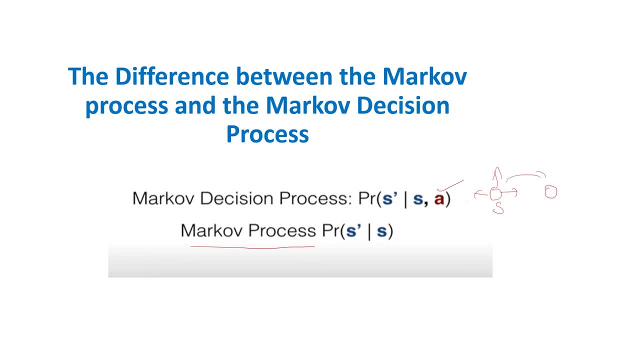 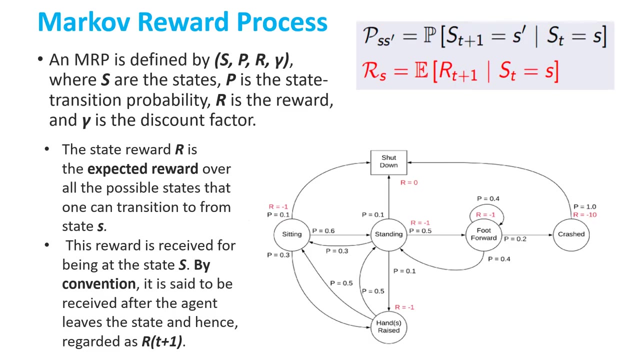 we can take while we transit from one state to another. so we are also interested in monitoring this action, along with the state transition probabilities. that is what Markov decision process is about. okay, so the rewards: this is the reward process is a four tuple: the Markov reward process defined by the set of states, the state transition probability, p. 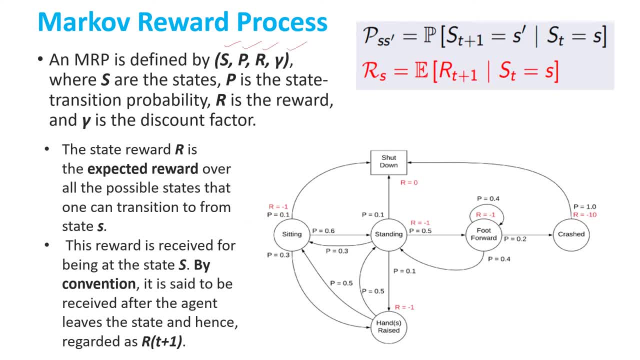 and the rewards that we get and the discounted factor. so the discount factor we'll understand better. we'll gain more clarity as and when we work out examples, but at this point of time, how this should be understood is that the discount factor is nothing but like how. 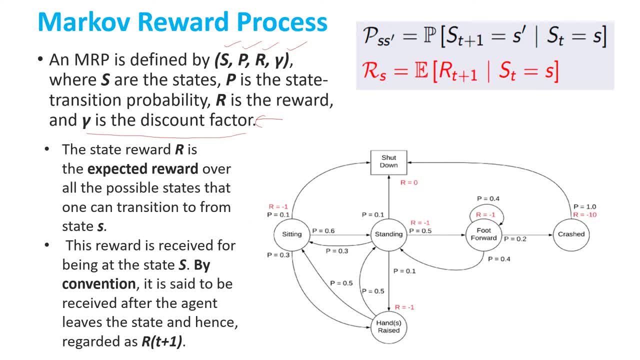 what is the importance that you give for the future? rewards, that is, expected rewards we do not know right, like when we are. when we are in one state, we might move to another state, but we do not know what is the reward that we get when we move to the other states. so we have some weighted 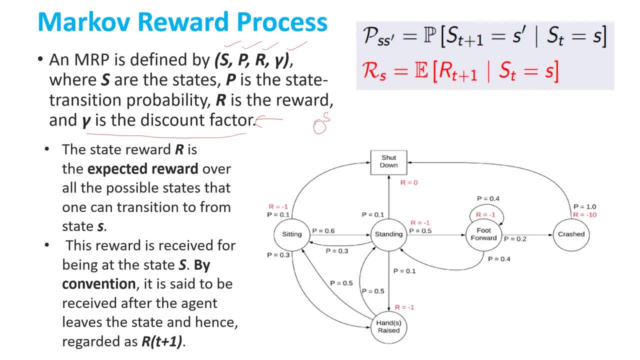 we give some, we give some weights to that, so that is discount. so at this point of time this could be understood this way. we'll gain a lot of clarity as and when we work out, with examples, the state transition. the same state transition diagram that we saw earlier is associated with the reward. 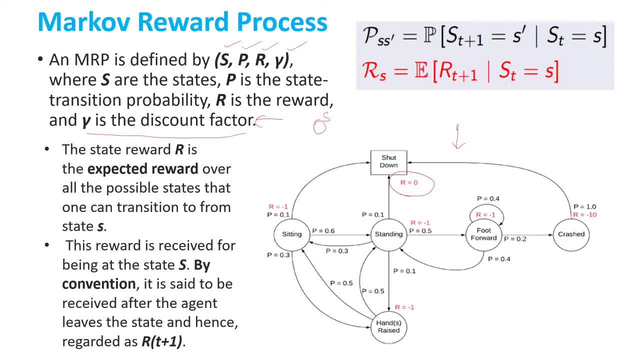 that is where this Markov decision process is gaining importance. like along the probability, state transition probability, we have also a reward- so that's what it says so from. while transiting from one state to s to s prime, so we get a reward also. so why we have it as t plus one is. 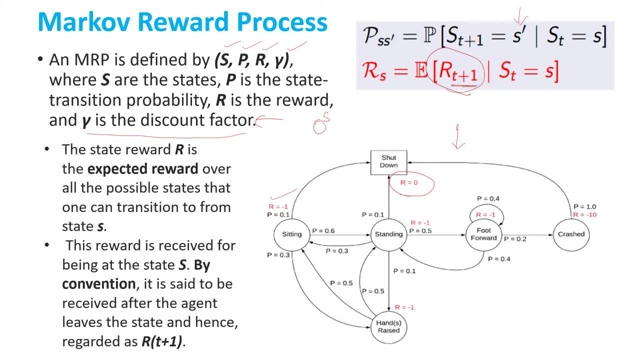 that. so this particular reward, r, is equal to minus one. is that so that an agent gets when it leaves from this state to any other state? so that's why it happens this and the. it is said that the the agent receives this award when it leaves the state, because that's why it is. 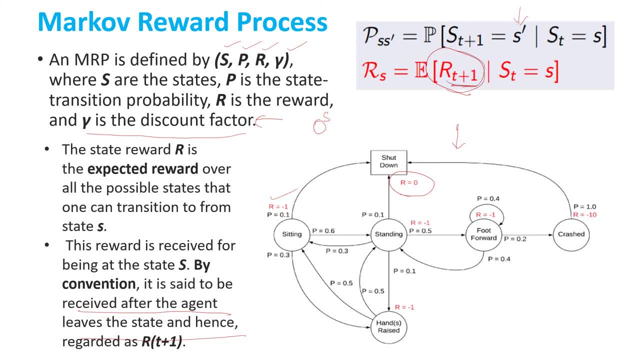 uh, taking at the time step t plus one. so that's why we have put it this way. so the probability that the reward function is as simple as this: when it transits from one state to another state, what is the reward it is supposed to get? so that's what we are interested in and our initial goal: that we 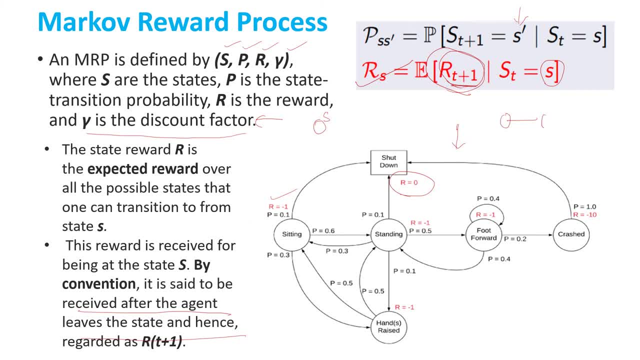 should remember, the agent is supposed to transit from one state to another state and consequent states to maximize the rewards. that's how it is aligning the action. that's why we are interested in finding what is the reward that we would get transit from one state to another. so that's where the marker process and the marker decision process. 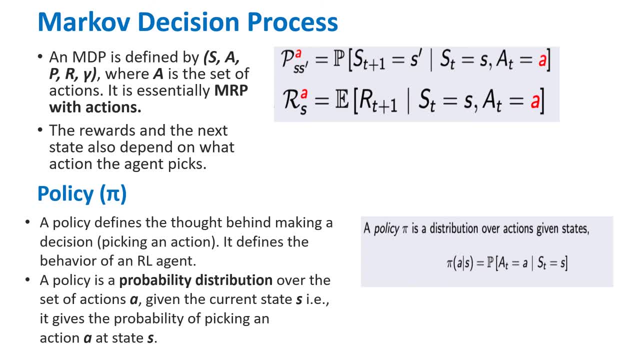 makes a difference. now we can understand an mdp. so mdp is a set of states and set of actions we take at each and every state and the probability associated with it, the rewards and the discounted factor, discount factor. so this is what is a mdp, so we can understand this. what is the probability? 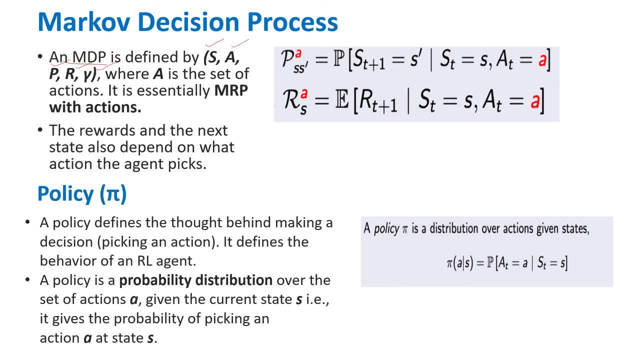 that, uh, the robot transits from one state, st to st, plus one, that is s prime, by taking a particular action. so why? because at each and every state we can have n number of action. so let's say we have go up, go down, or go right and go left. so these are four set of action. what is this? uh, small a. so what? 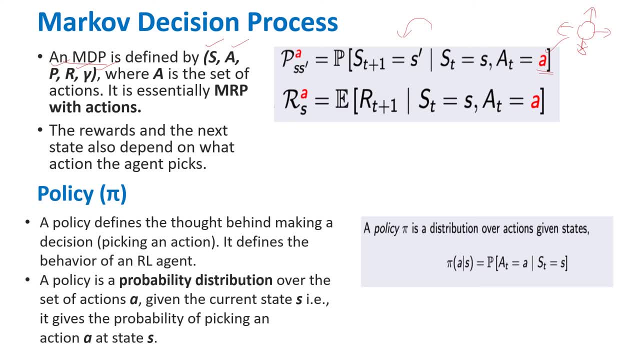 is the particular action, go right or go left. so that is taken from the set of these four actions. so that is also associated in predicting the next state transition probability. so that's how it should understood as: and the reward is the numerical value that we get when. 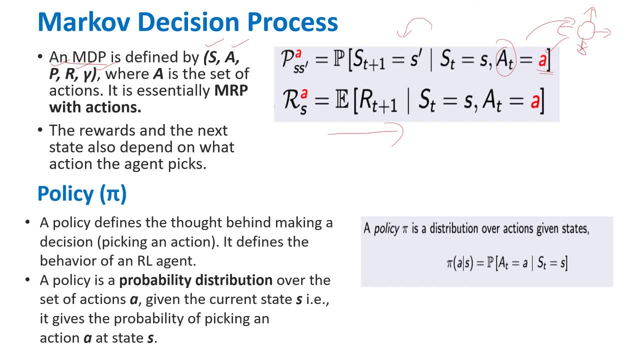 we do the state transition by choosing a particular award, uh, action, sorry. so the policy policy pi. so there's one more terminology: policy pi. so the policy pi defines the thought behind making a decision. it defines the behavior of an rl agent. so it's basically at each and 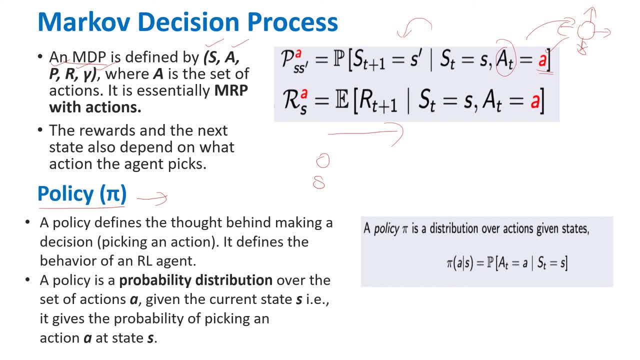 each and every state, we are taking an action right. so when we keep on transiting from one state to another, from each and every state, we are going to pick up an action right. so what are the set of actions we are taking? what are the right set of actions we are? 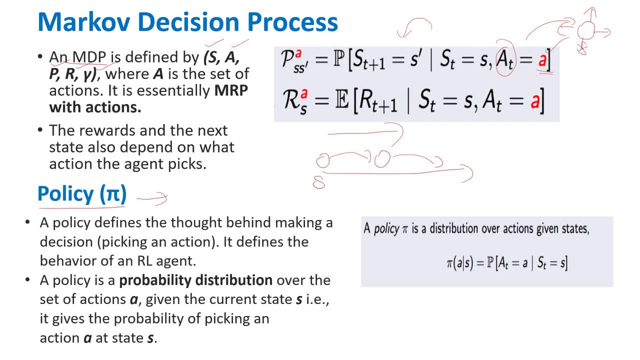 taking at each and every state, that string of actions. we call it as pi. so the pi can be thought of as a probability distribution over the actions given the states. okay, so, uh, it's a probability distribution from this particular state. what is the probability that you choose a particular action? what is the probability that you take right? what is the? 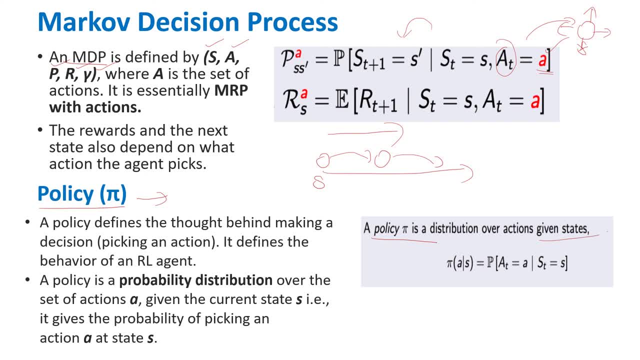 probability that you take left. what is the probability you take? you go up or go down. so that is policy pi. so it is also uh. can be thought of the um as a set of actions. we are bothered about, like choosing the right set of actions that should be chosen for each and every state when we transit. 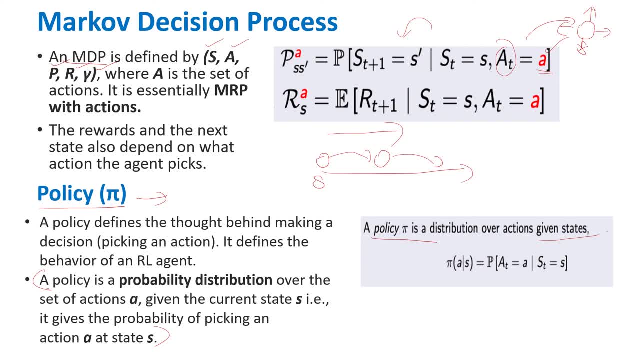 from one state to another, depending upon the reward. so there are three things that should be understood. uh, we are taking a state transition from one state to another and we are doing so. we are keeping in mind of the rewards that we are collecting and also we are also taking into 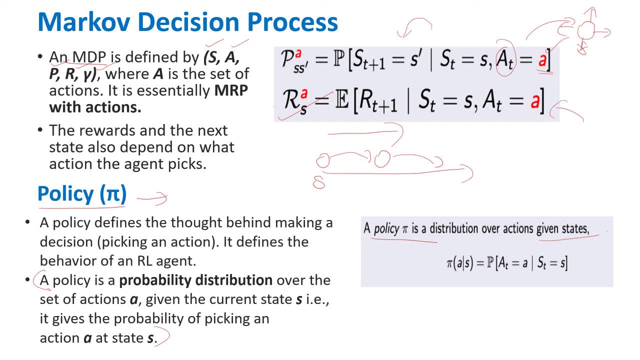 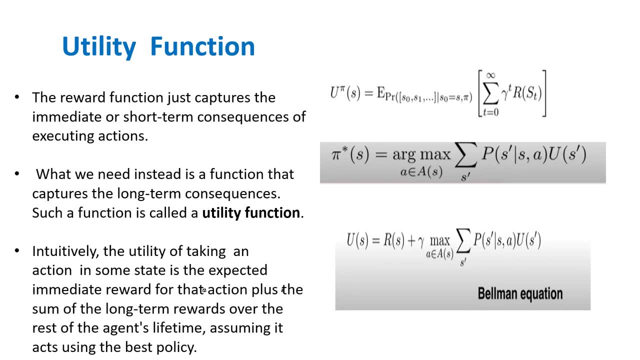 account the actions. so what is the right action that would maximize the reward? so actions, reward and the state transition, so three things that should be kept. there's one more function. we have utility function, so the reward function is only bothered about like, what is the reward that we? 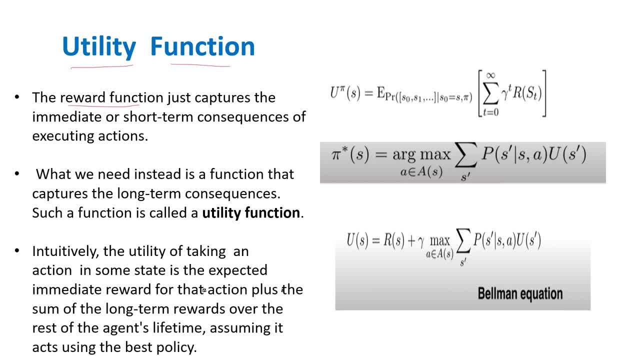 get when we transit from one state to another. so but we are interested in the overall uh. our vision is to reach from the starting state uh to the final goal right. so when we are doing so we will have n number of state transitions in between, and when we will have the rewards and we will 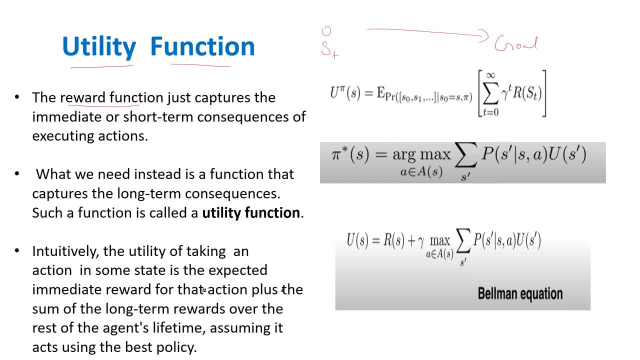 choose each and every actions. what utility function is bothered about is that. you see a pie here, right? so we are bothered about the policy. the policy is all about choosing the actions. so the utility function is for a particular policy. there can be a number of policy, but for a particular policy, what? 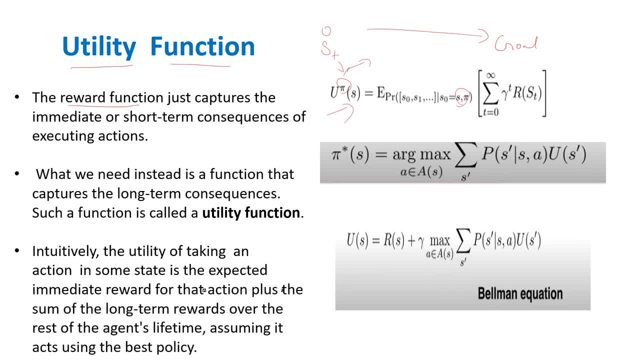 is that? so we are in state? yes, right, and we are. what is the probability that we will go to these set of states for using this policy pi? so policy pi is nothing but the set of actions we take. for instance, we are in state starting state, we will move right. 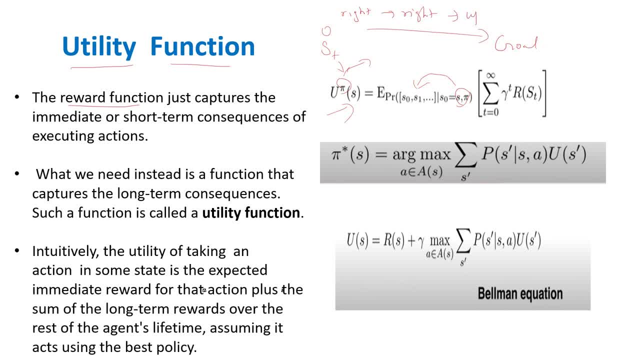 and then we will take a right, go up down. so this is a policy, pi so, and then we reach the goal. so this is one policy by one, so there can be a number of policies. so for this particular policy, what is the expected probability of transiting from these states to? 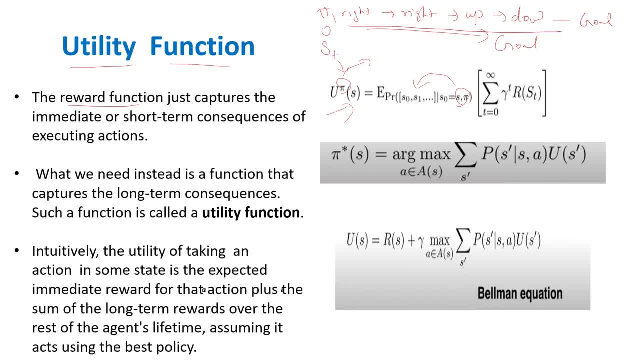 another, multiplied by the sum of, uh, um, the discounts. so this is the weight factor we were talking about. so this is a prediction. so what is the reward that you would get when you land in the con consequent states? that's what we are bothered in. so this is indirectly, this equation is telling us. 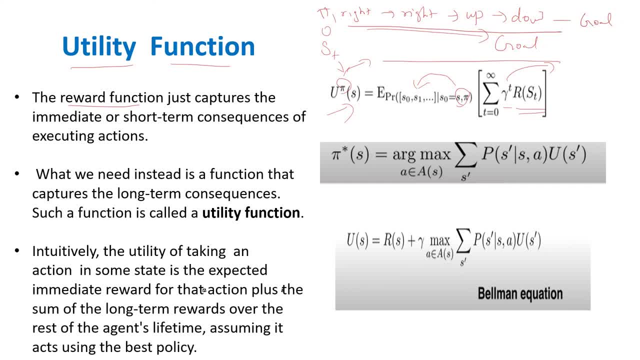 that we are supposed to maximize the rewards whenever we take a transition from one state to another. so that's the goal, so that's the utility function, because there can be a number of policy, there can be a number of sequence of actions that you might take while you take a. 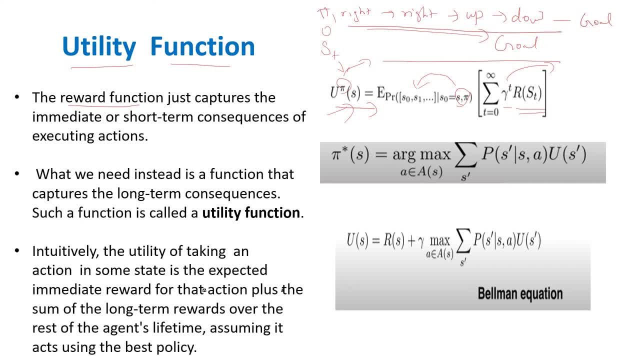 state transition, but you might also- you might also like- have to monitor the rewards you get while you take a state transition. that is the pi of s. so the pi of s that is- uh, i'm sorry, that was- utility function, u of s. and the pi of s is nothing but the policy, the policy we are. 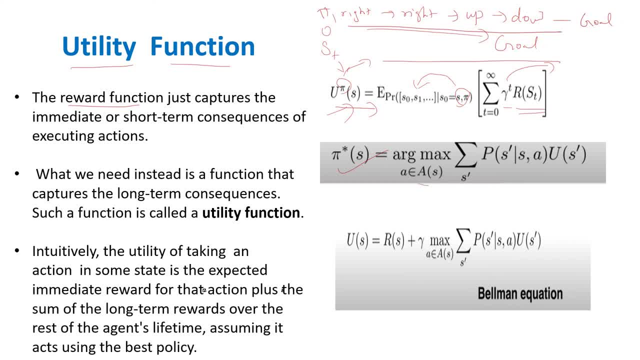 interested in. so that is the maximize there are a of s is the set of actions that you take from each and every state and what is the right action you take. so at each and every state we are, we have this utility function and the probability of state transition. 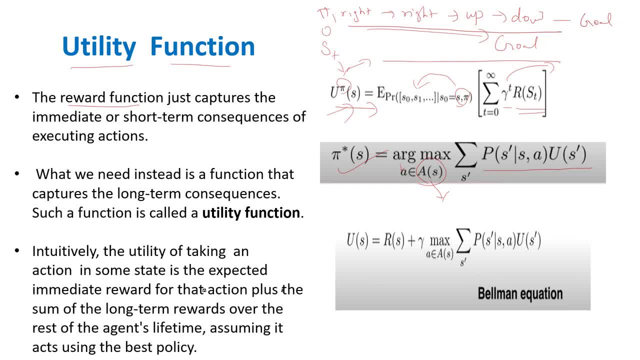 but which action gave you the maximum utility value? so that's what this equation is telling us. so, whether the go right action is giving you the maximum value or the go left action is giving you the maximum value, or go up or go down, so which was giving the maximum value? so that's how we align. 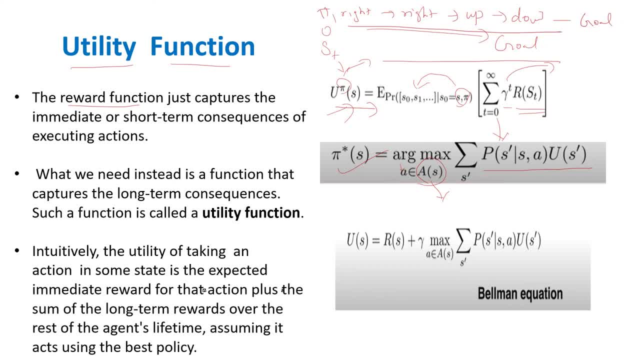 the set of actions we take at each and every point of time. so the utility, uh, the utility function in general. so this is a bellman equation, actually. so utility function of a particular state is not nothing but the reward that you get at that particular state plus, uh, the discount factor. 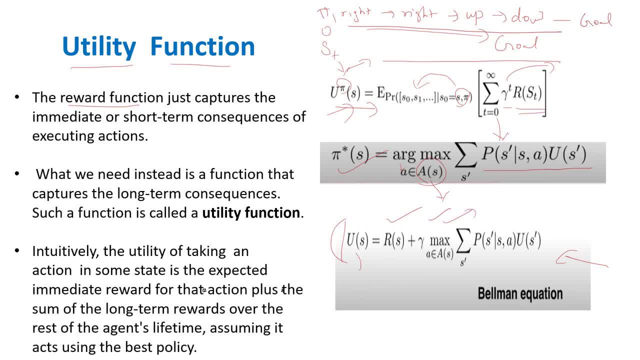 multiplied by the maximum probability. so you take what is the policy that you gave that gave the maximum uh utility value. so this is a prediction. this is s prime is got from the future States. that's how we'll understand. we'll understand all this when we work out an example in upcoming videos. 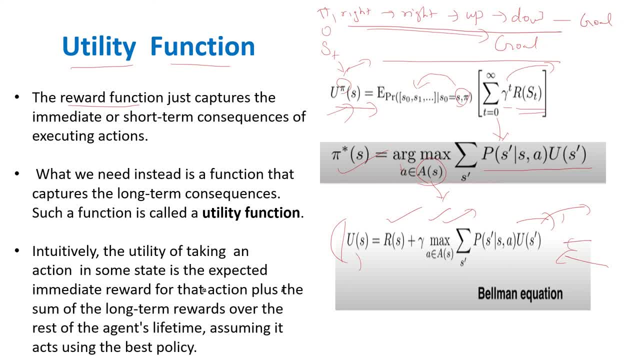 but as of now it can be thought of this. so, while we take a transition from one state to another, what is the right action we are supposed to make? That's what utility function and the policy pie is telling us: Okay, so this is an. 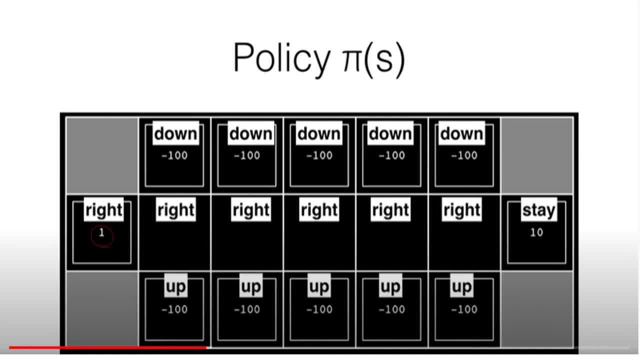 example policy that we see. So you see here this is one goal state and another goal state. So a good agent is supposed to reach this goal 10,. right, Because that is having the maximum reward. So we are not supposed to tuck here. So these are the policies you see. So let's say the agent is 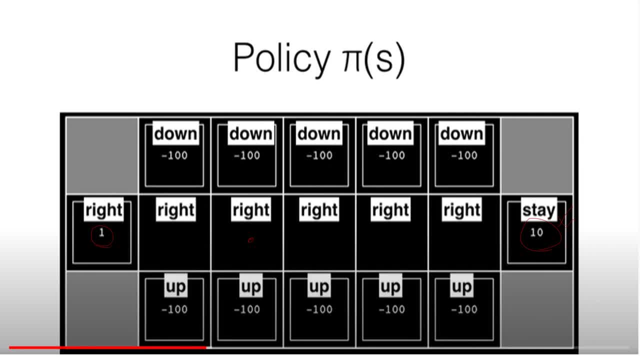 here. So then if agent can land in any state, right, So random, it's random. So let's say we are in this state. Then this state says that the policy is right, So we are supposed to move this way. So this state also says that it move right. This state also says that we should move right. 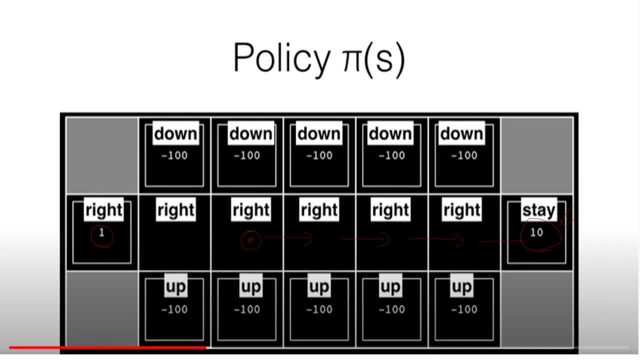 And this state says we should, Because we have achieved the maximum goal, we can settle here. Let's say, if we have landed here, then it says that okay, this is not the right place You are supposed to go down And from here. 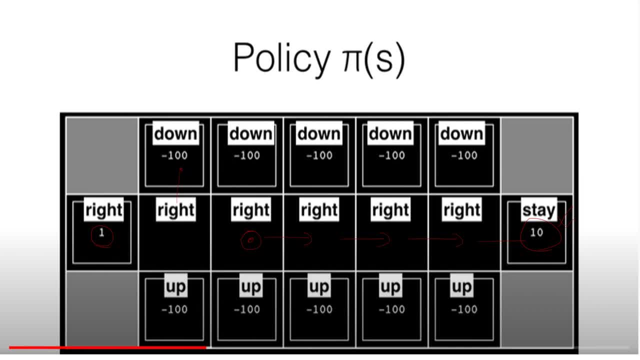 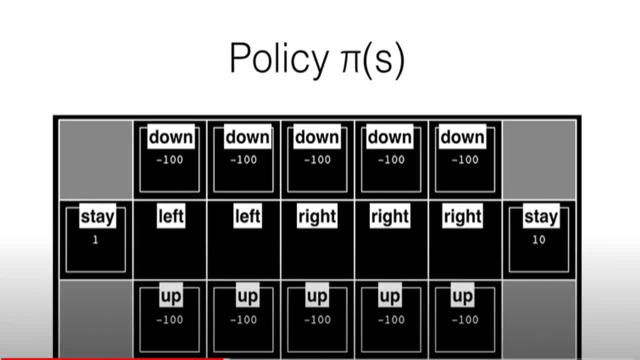 we will move right. This is a good policy. So this is the best policy the agent has learned on its own. But if you see here this is a bad policy, Maybe the agent has learned this bad policy in initial state And as and when the training, the time moves on, it will learn the best policy. 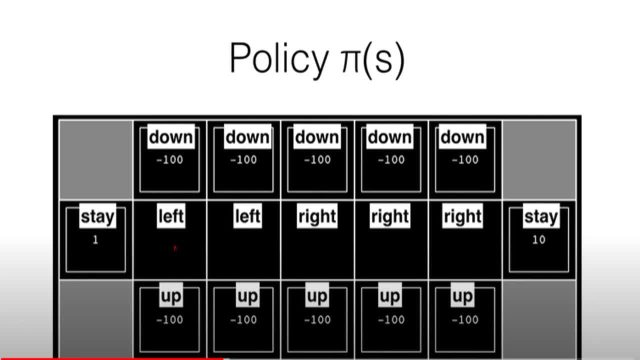 See here, if you can see here, if the agent is here, it says that it should move left And this says that it should stay. It's not supposed to stay right, Because the maximum goal is staying lying here, So it should have been right here. So we should have, instead of stay, the action. 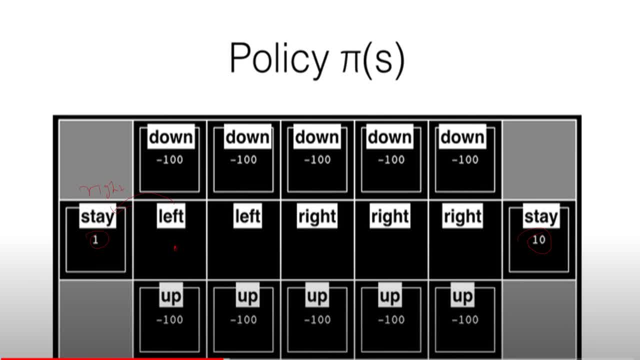 should have been right. So then only we can move it here, So move towards this state, And this should have been right instead of left. Then only we can move, So we can align our, our actions. So this policy is a bad policy. Maybe this was an initial policy. 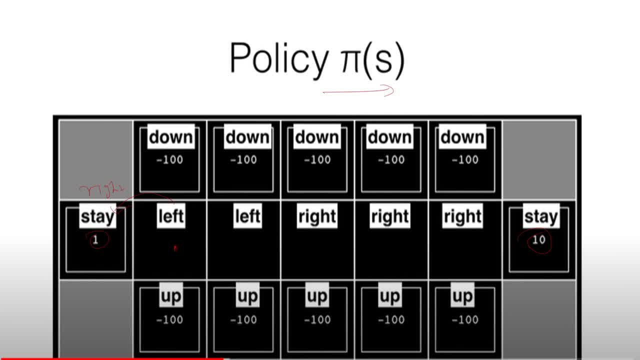 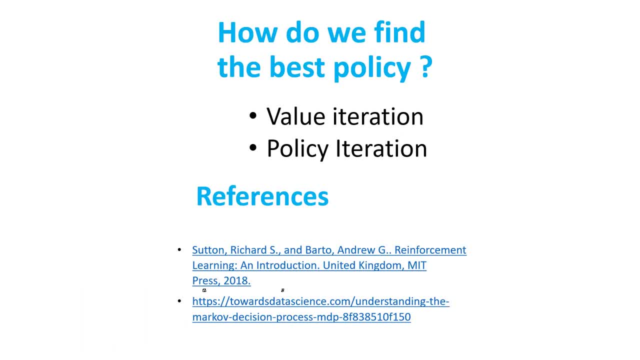 learned by the agent. So, but the reinforcement learning is all about like learning the right policy over the period of time. Yeah, How do we know that we learned the best policy? How do we learn the best policy? There are techniques to do that: value iteration and policy iteration. So we